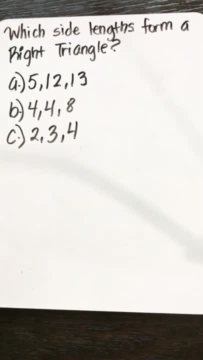 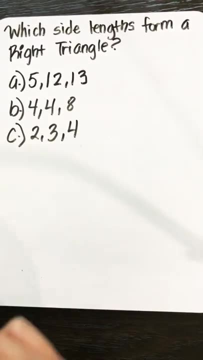 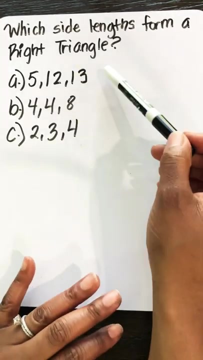 Hey guys. so I'm gonna do an example that is directly from Khan Academy, just so that you all know how to do problems like this. So this question is asking which side lengths form a right triangle. So A, B and C, are both or all three the 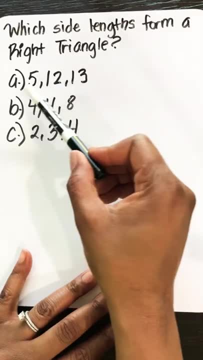 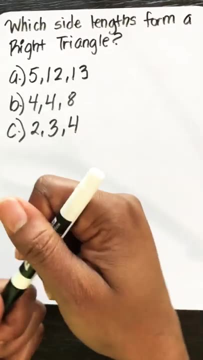 length of a sides of a triangle. So they're saying: if these were the length of the sides of each of my triangles, which of them would be an actual right triangle? Okay, so the best way to do this is you want to take each one, so 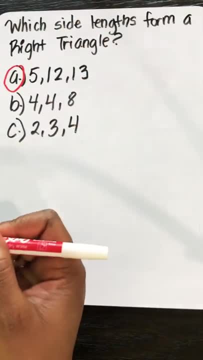 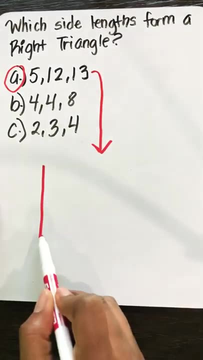 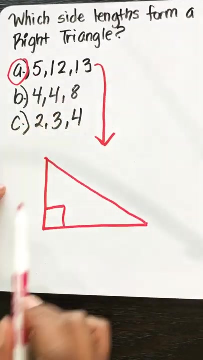 let's start with A, and you want to test it out using the Pythagorean theorem. So if we were to test it out, we want to first draw our right triangle right, So we've got a side length of 5,, 12, and 13.. Well, looking at these numbers, which of 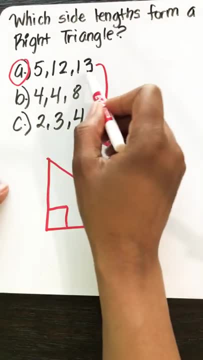 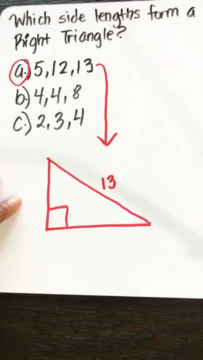 those would be your hypotenuse. Well, remember that our hypotenuse is our longest side, so that means that 13 would be your hypotenuse, because that is the biggest number. And so that leaves our other two numbers, 5 and 12, as the length of our legs, And again, it doesn't. 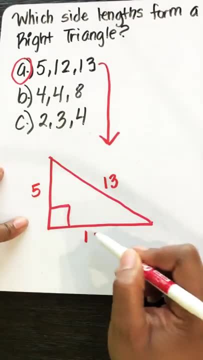 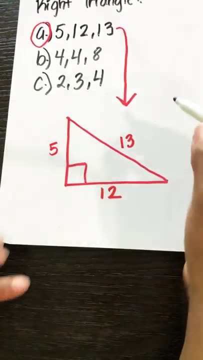 matter which one, but I'm just gonna make the shorter one 5 and the longer one 12.. Okay, so now we have labeled the sides of our right triangle and remember that your hypotenuse is C and your two legs are A and B. 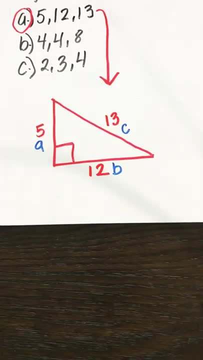 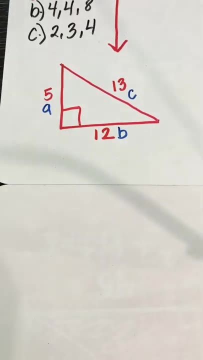 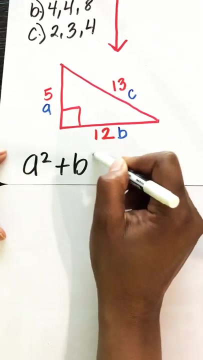 So what we want to do now is we just want to test out each of these numbers to see if the Pythagorean theorem is true. Okay, and I'll explain what I mean. So remember, the Pythagorean theorem says that A squared plus B squared equals C squared right. So what we want to do is: 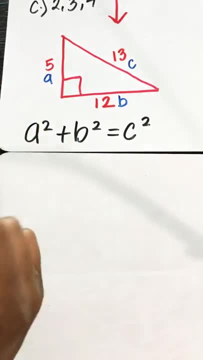 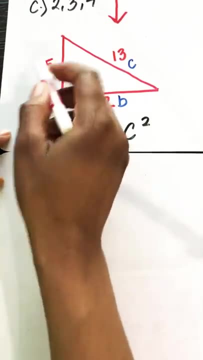 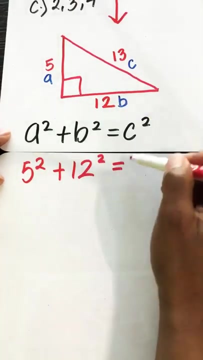 we want to take our A square it, Take our B, square it and then take our our c and square it. so if we start with our a, that would be 5 squared, our b is 12 squared and then our c is 13 squared. so all we've done is we've taken our values and just plugged it. 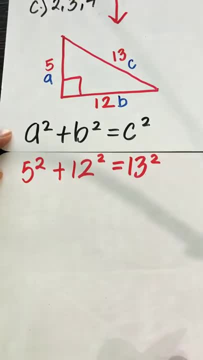 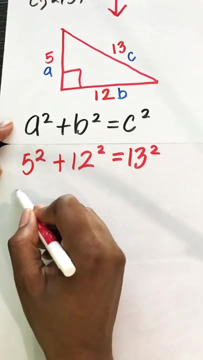 into the pythagorean theorem. so now we want to check to see if it's true. okay, and what i mean by true is if it's, if they're going to be equal to each other. so 5 squared is 25, 5 times 5. 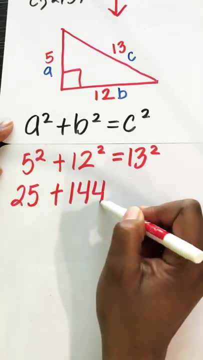 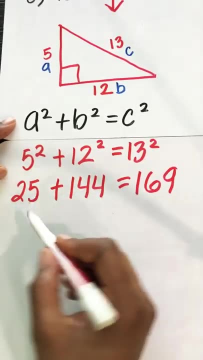 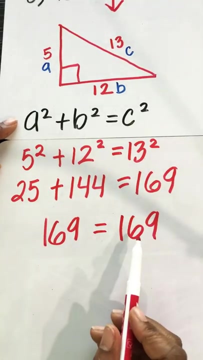 12 times 12 is 144, 13 times 13 is 169, and then we want to add these two together, this would give us 169. okay, so now we have completed the equation and, as you can see, we have a true statement here, because 169 equals 169 and because we created a true statement, we can go back to our original. 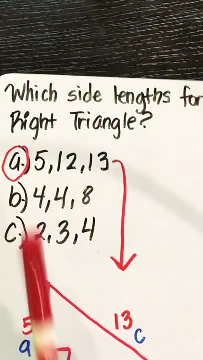 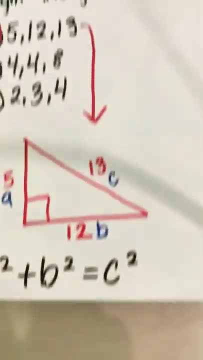 statement and we can go back to our original statement and we can go back to our original set of side lengths and say that a is a right triangle. how do we know? because we tested it out on pythagorean theorem and we got a true statement. if you were to test out, let's say: 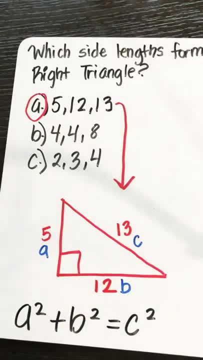 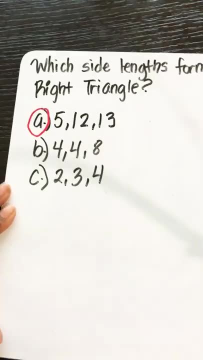 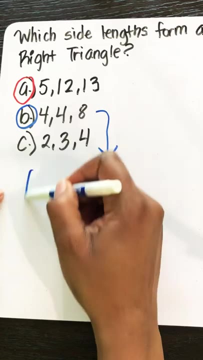 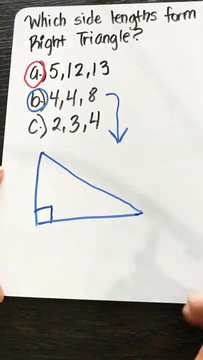 let's go ahead and test out b, okay, just to see what will happen. let's test out b and see what happens. so we're testing b- the side lengths for four and eight, right? so again, we're going to draw our right triangle, label our sides, okay? so we know that our hypotenuse is the longest side, which means 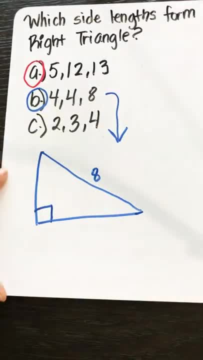 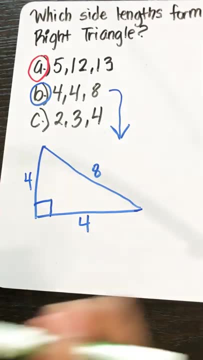 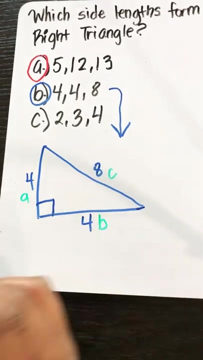 our hypotenuse is going to be eight, and then we've got four and four. so it doesn't really matter which ones we label four and four. so again, remember, hypotenuse is c, um, and then we've got a and b. so we're going to test it out, and we're going to test it out, and we're going to test it out. 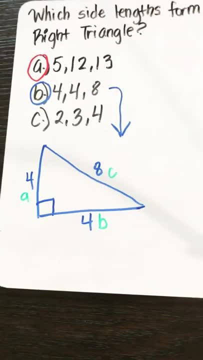 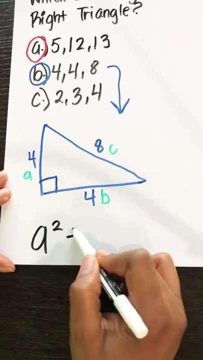 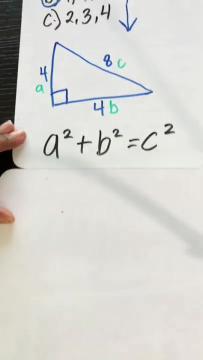 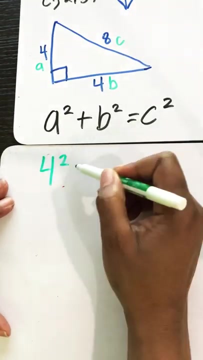 pythagorean theorem, again using these numbers. okay, so we've got a squared plus b squared equals c squared. so we're going to take our values and plug them in. so we're going to start with a squared, which is four, so that's four squared plus b squared, which is four squared again.